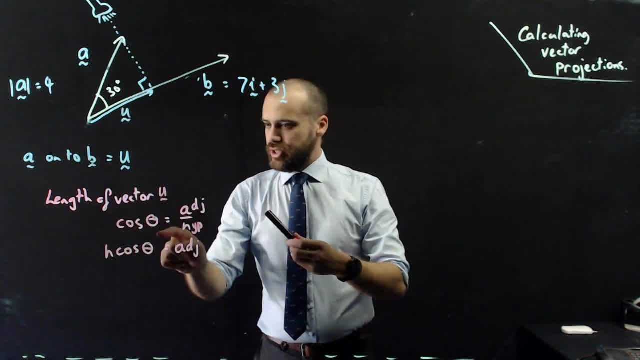 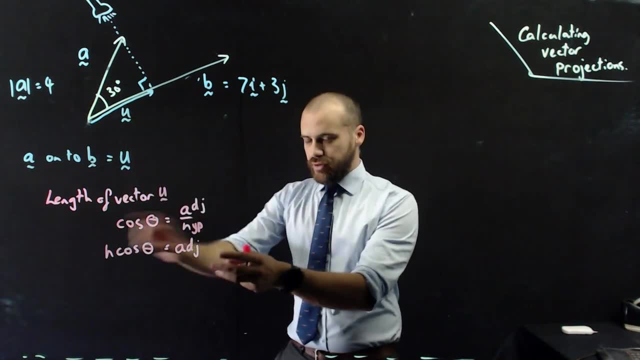 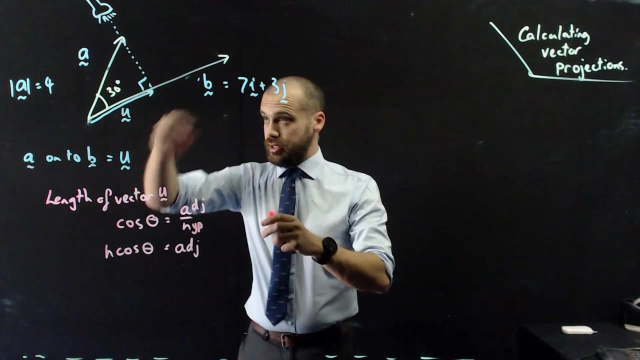 length of vector u in this case. Now cos theta adjacent over hypotenuse, cos theta equals adjacent over hypotenuse and we can rearrange that to say that hypotenuse times cos theta equals adjacent. now, in this particular question, the adjacent is this length, here which 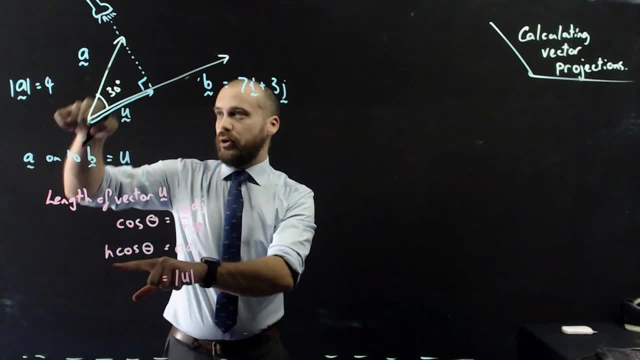 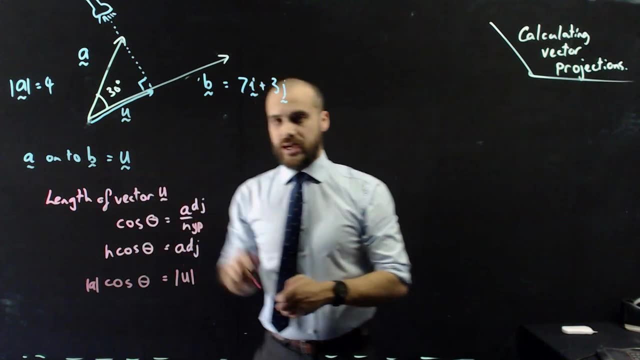 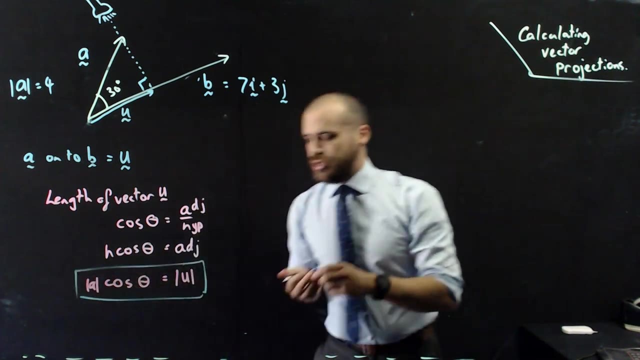 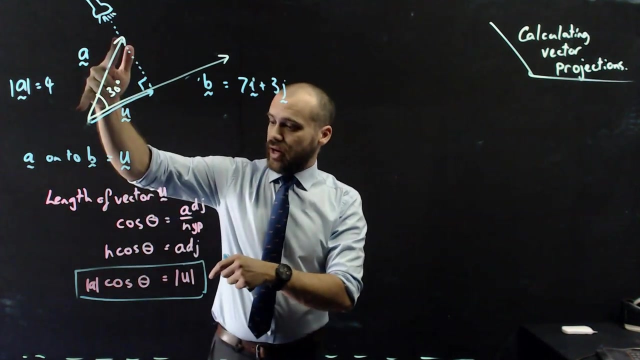 is the magnitude of u, the hypotenuse is the magnitude of a and cos theta is obviously cos theta the angle here. all right, that piece of information is really important. so that says that the length of the vector projection of a onto B will be equal to the magnitude of a times the angle between a and B. 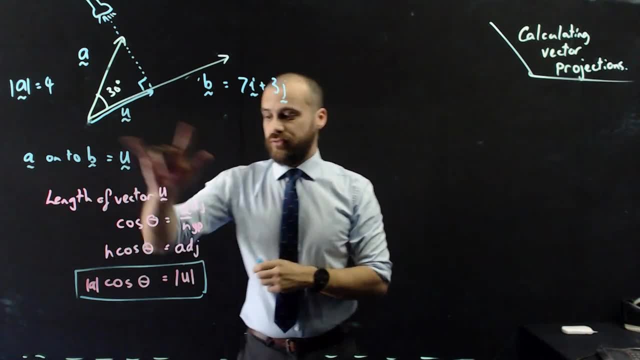 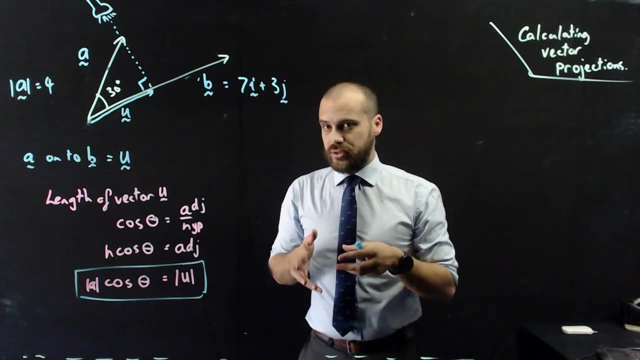 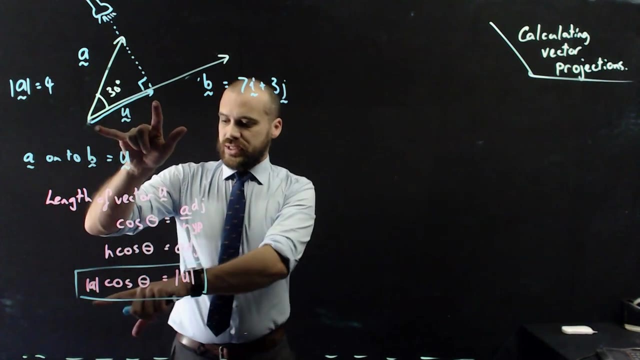 alright, so now that tells me the length of vector u. all right, I'm just going to hold that there for a second, because I don't want to know the length of vector u. i want to know vector u. i want to know what it is. so it's this length in vector b's. 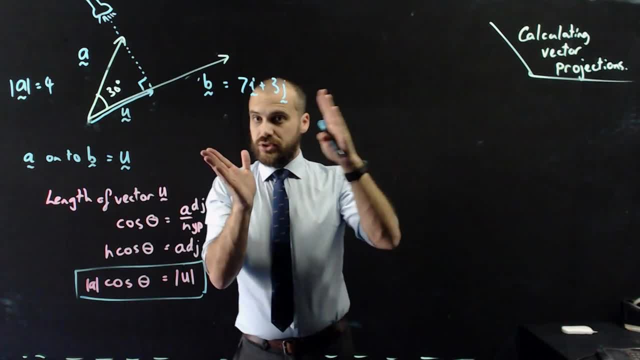 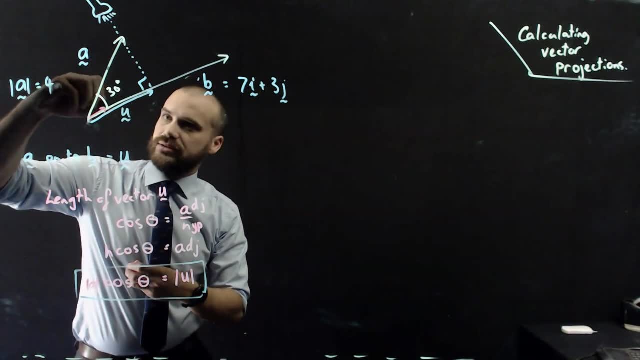 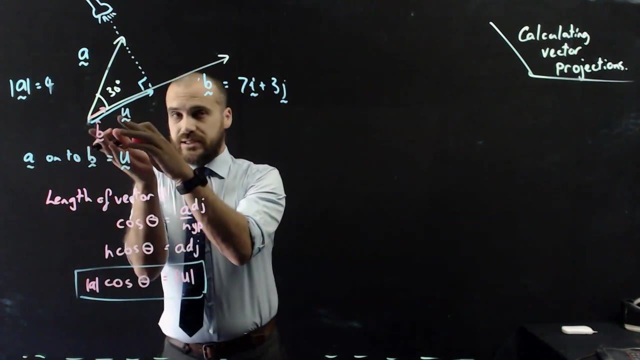 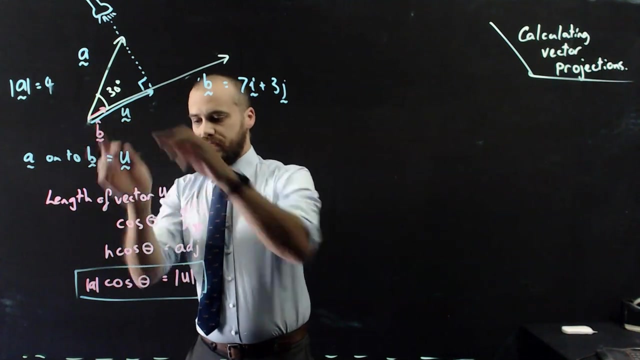 direction. so if i find the unit vector of b, that'll give me a tiny, tiny little vector here called the unit vector of b. so i scale that down and then, if i've got the unit vector of b, i can then multiply whatever, the whatever that is, by that length, and then i'll scale it back up. 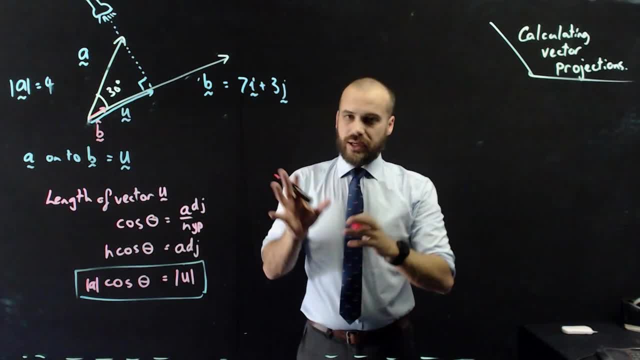 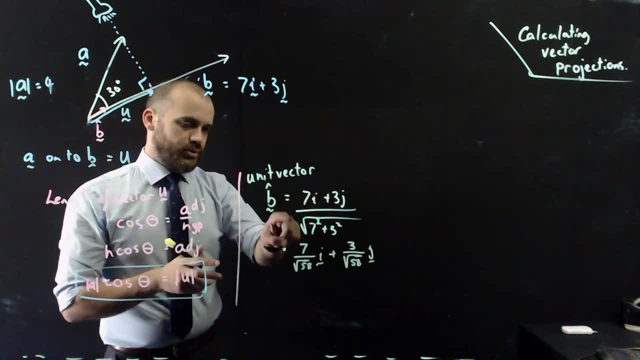 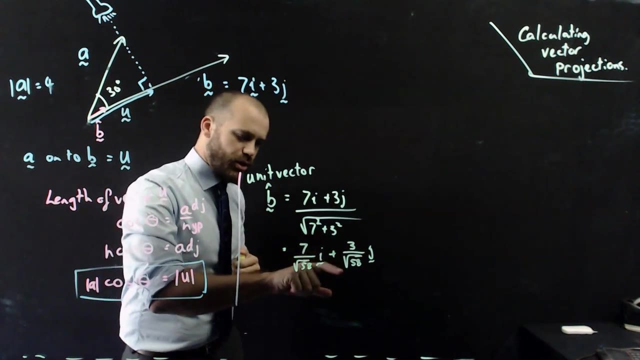 and i'll have an answer. all right, seems a bit bit wacky, but let's do it. so the unit vector of 7i plus 3j is 7i plus 3j over the magnitude of b 7i plus 3j, which is 7 over root 58i plus 3 over root 58j. that's this little pink thing here which. 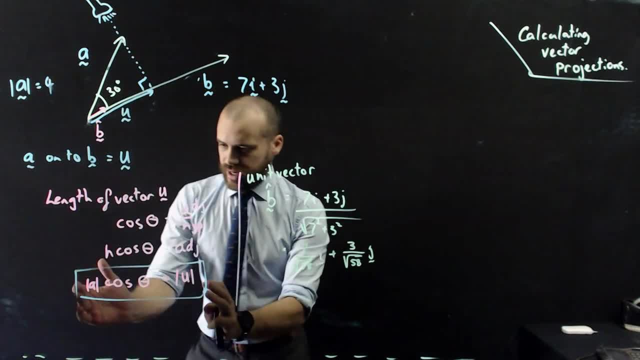 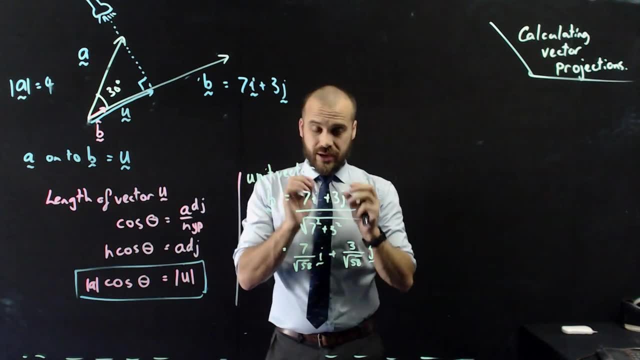 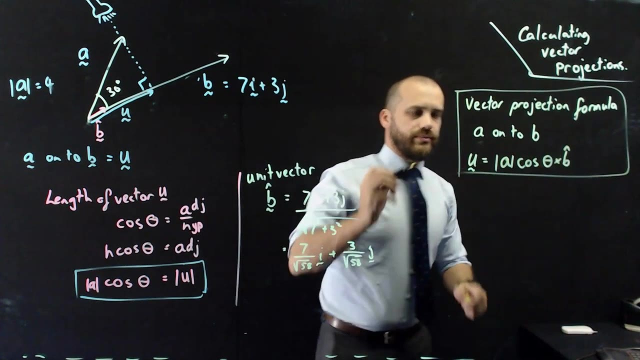 is the unit vector. now i need to take that length, i need to multiply it by that and i'm going to have my vector projection. here is our vector or one vector projection formula. vector projection formula. important information: if we're projecting a onto b, we'll get a. 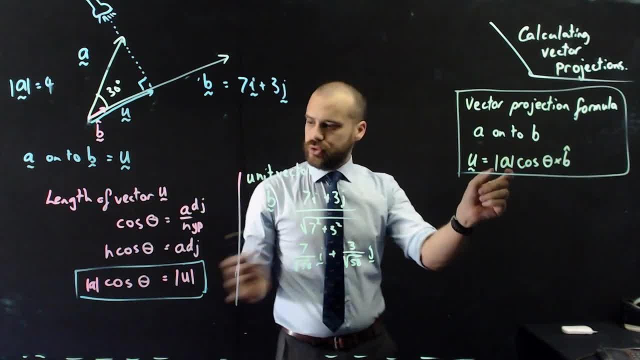 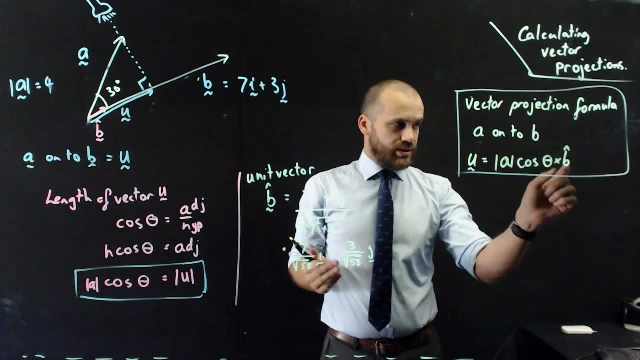 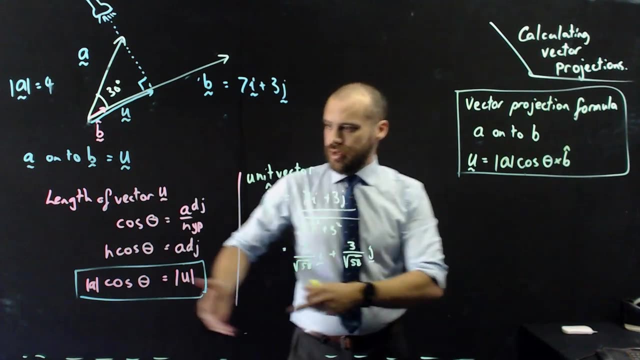 vector called u, which is arbitrary. it's going to be equal to the magnitude of a cos theta, because that'll give us the length of it, and then, if we multiply it by the unit vector, we'll get the components i and j. all right, so we can finish off our example here by taking whatever that value is. 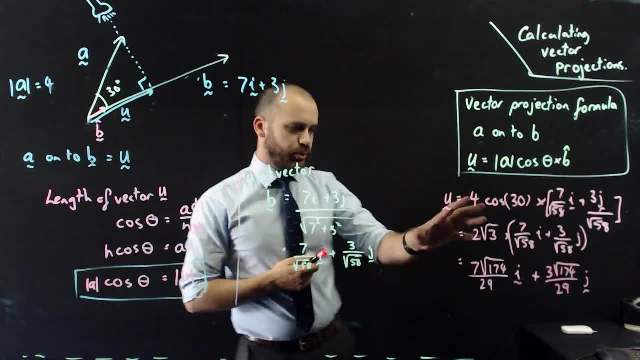 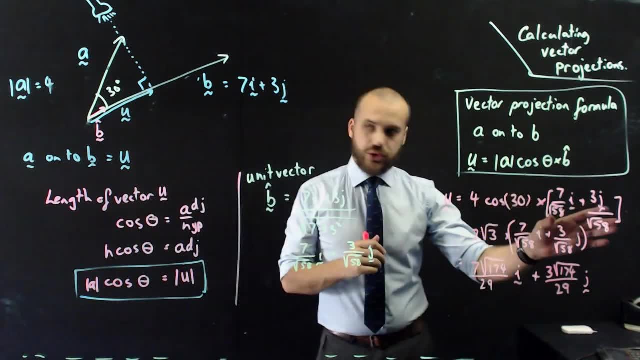 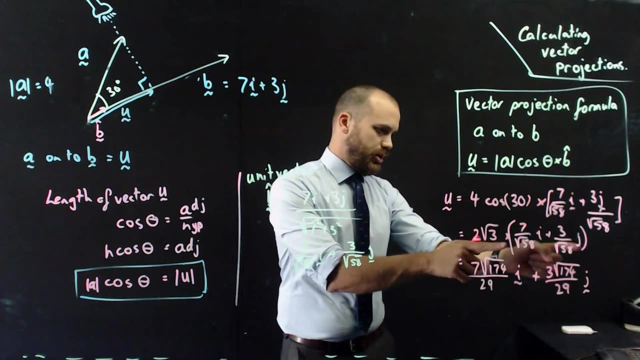 multiplying it by that value and getting an answer. so here i've put it into my formula: four, which is the magnitude of a times cos theta, which is the angle between them, times the unit vector of b, and then four cos 30 is two root three. two root three times the unit. 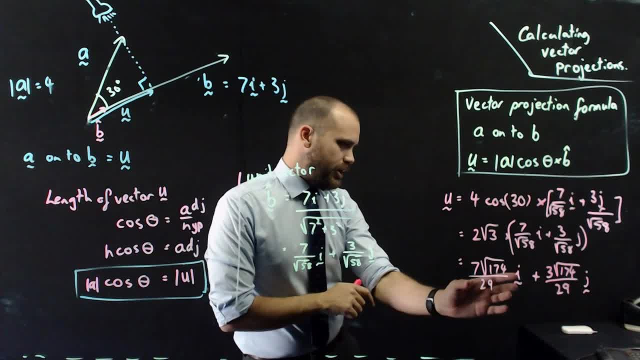 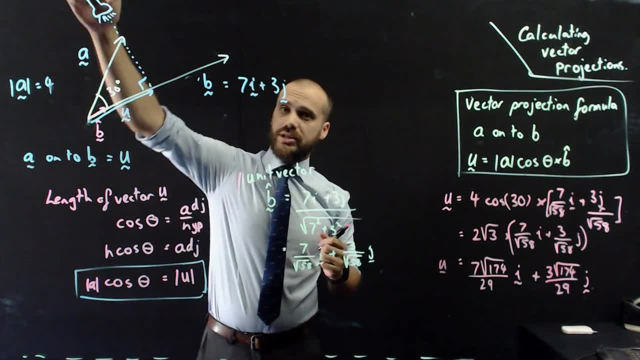 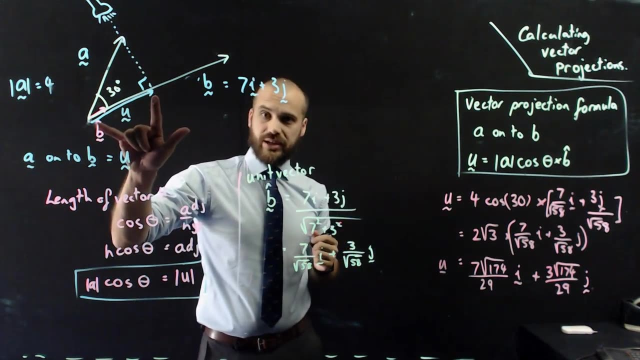 vector of b and we get our answer in terms of i and j. now again, what is that? that's the vector, that is the shadow. when a torch is put perpendicularly to vector b and creates this, that is that vector there. now, that is a good. 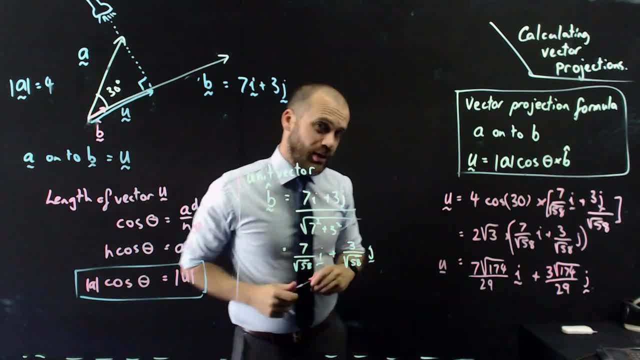 there now that is a good there. now that is a good formula for the vector projection. but there is another neat little one that I want to show you that we can sort of prove from that Now you might have noticed when you were doing this that 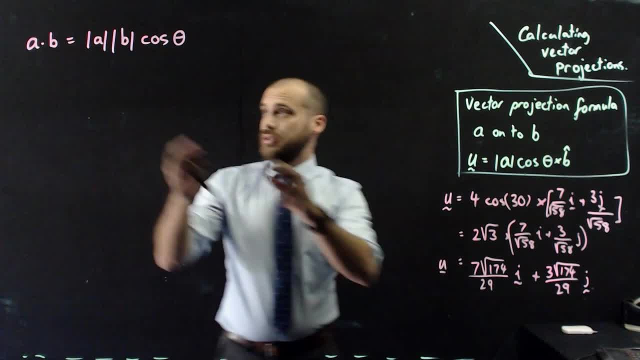 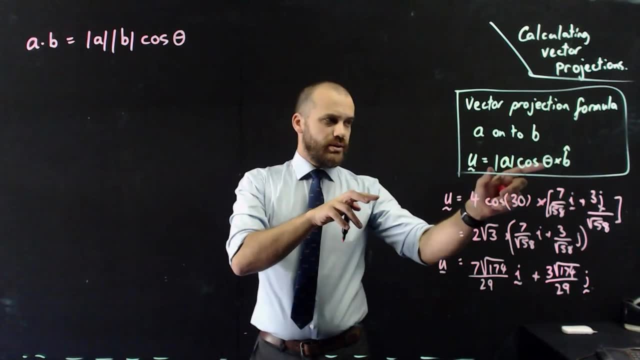 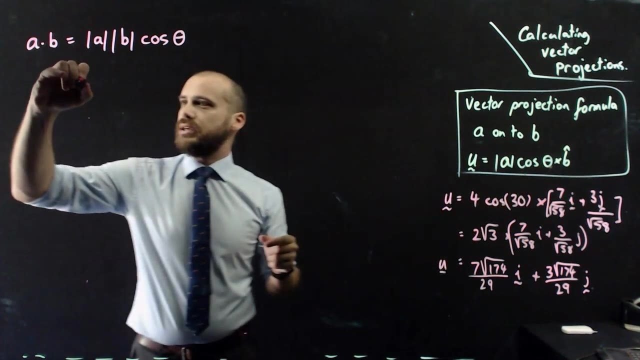 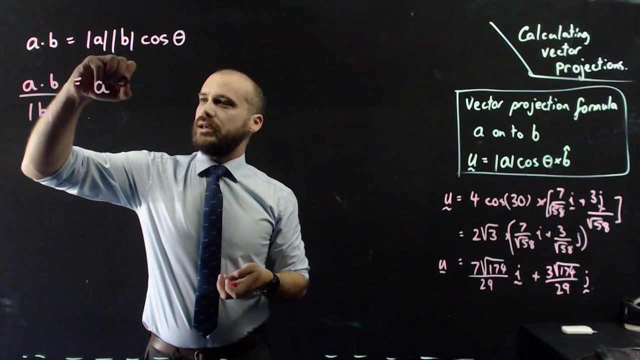 a cos theta is part of the dot product formula a, b cos theta, magnitude of a magnitude of b cos theta. So I'm going to just figure out how to make that something else. Now. if I divide by the magnitude of b, I get a dot. b divided by the magnitude of b equals a cos theta, That seems. 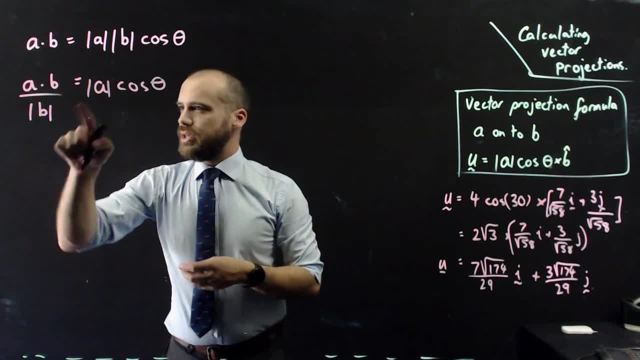 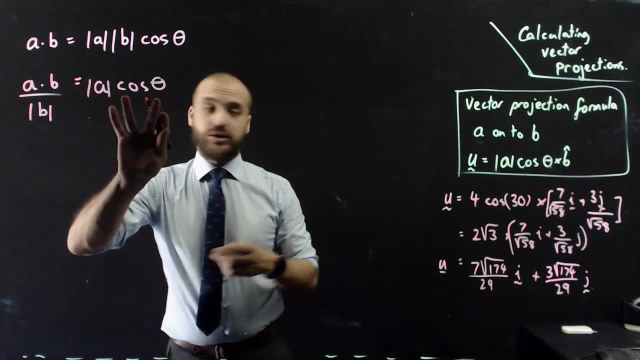 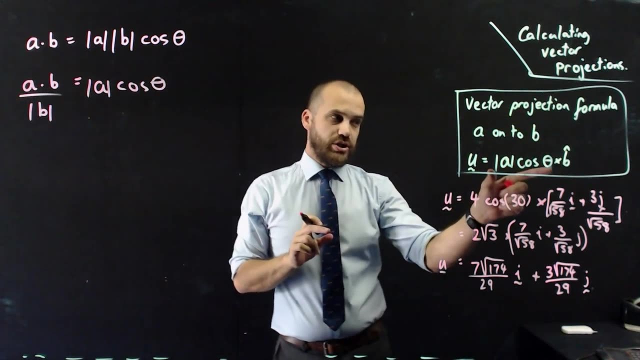 useful to me. I can now say that a dot b over the magnitude of b equals the magnitude of a cos theta. So I could, if I wanted to, take that thing there and shove it into my vector projection formula. and now I've got a new vector projection formula. that is kind of useful. 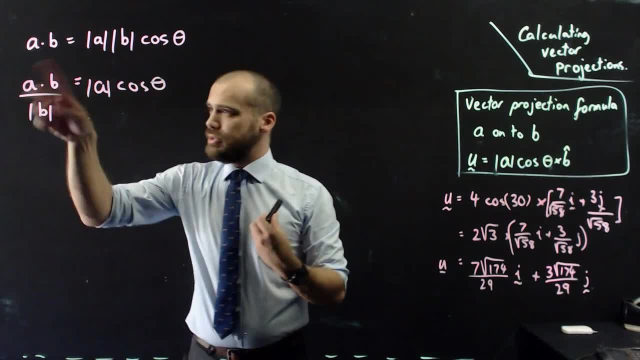 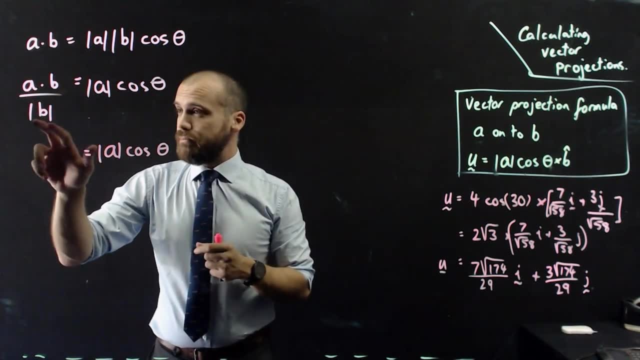 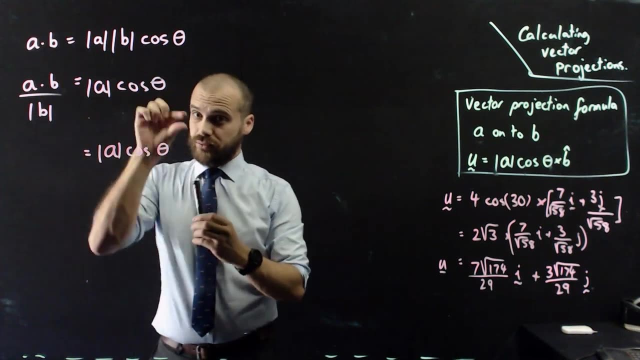 because it doesn't use an angle. But I can simplify that just a little bit further. If I take a vector b and divide it by the magnitude of itself, I get a unit vector. So I can rewrite this little formula in a little bit of less work: Vector a dot vector b.